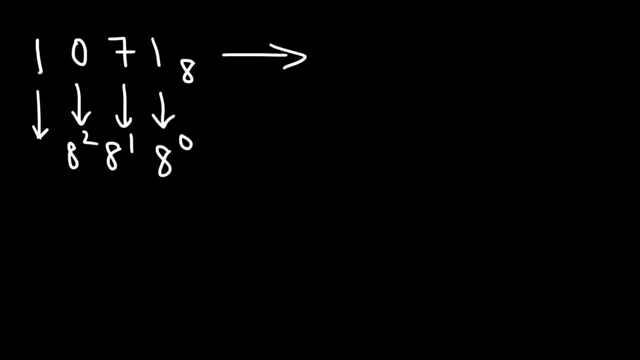 the first power and the 0 by 8 squared and the 1 by 8 to the third. So this is going to be 1 times 8 to the third, plus 0 times 8 squared, plus 7 times 8 to the first power, plus 1 times 8 to. 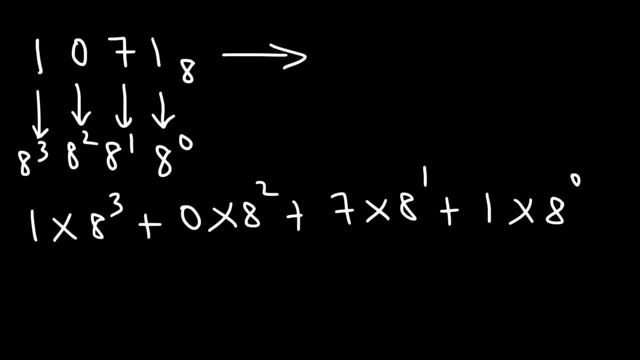 the 0 power. So what is 8 cubed? So 8 times 8 times 8, that's going to be 512.. 0 times 8 squared is 0,. 7 times 8 is 56, and 8 to the 0 power is 1.. So 1 times 1 is 1.. 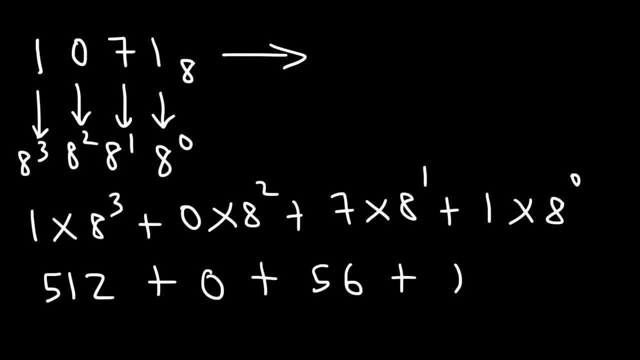 So we have 512 plus 56 plus 1. And that's going to be 569 in the base 10 system. And so that's it. Now, what about this one? 16,475 in the octo system? Let's convert it to a decimal number in the base 10 system. 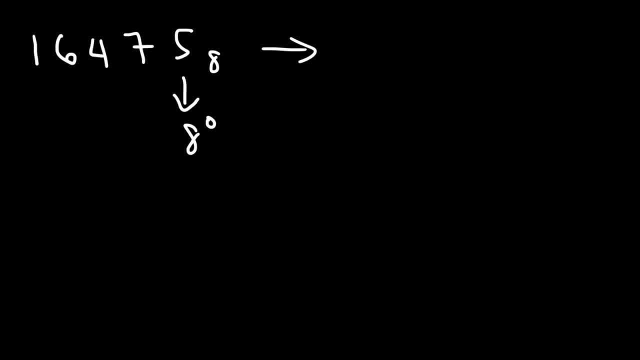 So the first number, the 5,, we're going to multiply it by 8 to the 0, and the second number by 8 to the 1, and the third by 8 squared, and the fourth by 8 cubed, and the last one by 8 to the fourth. 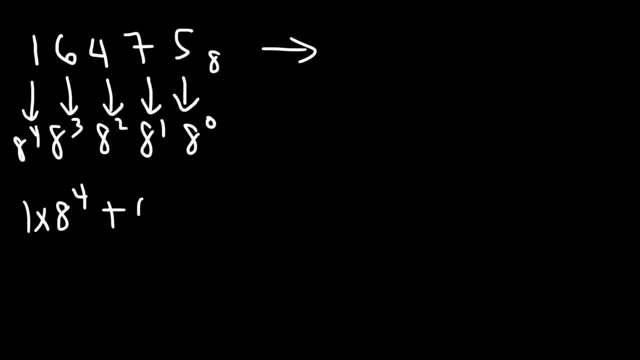 So this is going to be 1 times 8 to the fourth plus 6.. 6 times 8 cubed, plus 4 times 8 squared, and then plus 7 times 8 to the first power and then plus 5 times 8 to the 0 power. 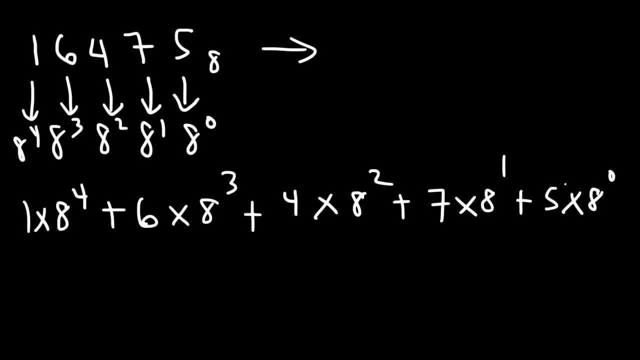 Now 8, raised to the fourth power, if we multiply 4- 8s together 8 times 8 times 8 times 8, that's 4096.. Now 8 to the third. we know it's 512.. 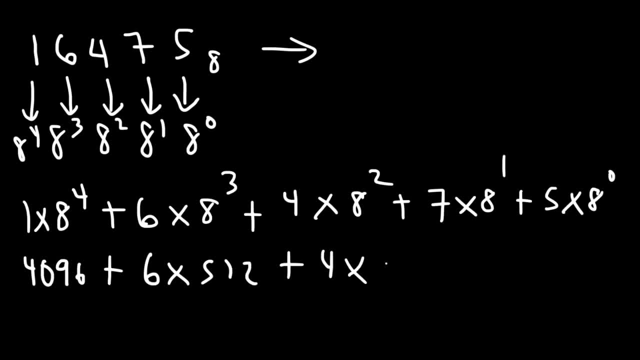 And then 8 squared is 16.. 7 times 8 is 56, and I need to put a plus sign here- and then 8 to the 0 is 1.. So we have 4096, and then 6 times 512,, that's 3072, and 4 times 64 is 256, and then plus 56, plus 5.. 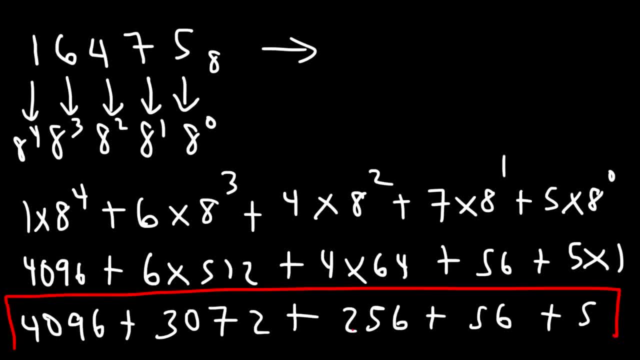 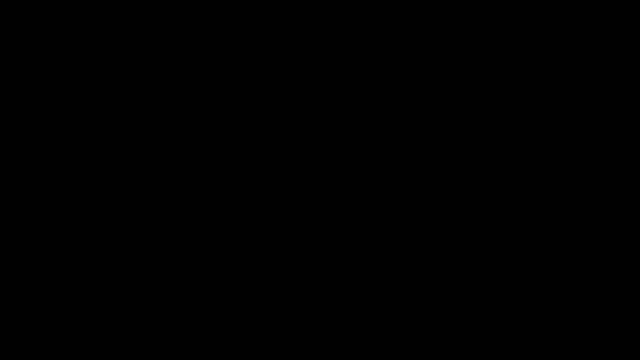 So let's go ahead and add up these five numbers, And so the sum comes out to 7485 in the base 10 system. So this is the final answer. Now what if we have a fractional number, Let's say 425.28 in the octal system? 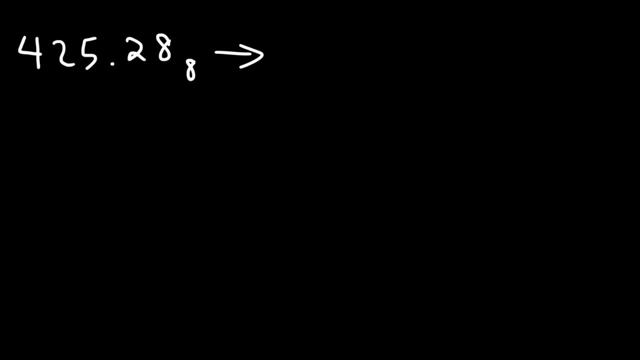 How can we convert that to a base 10 number in the decimal system? So we know that the 5 we need to multiply by 8 to the 0, and the 2 by 8 to the 1, and 4 by 8 squared. 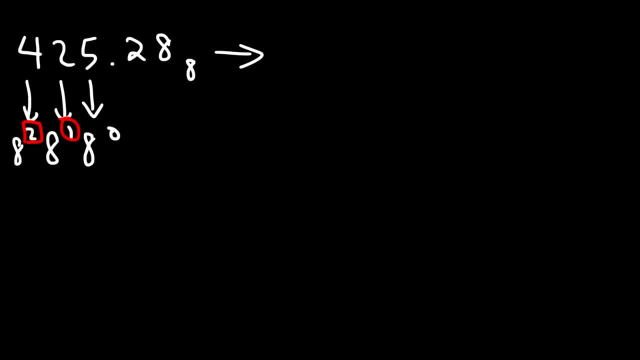 So if we follow the pattern of exponents that we see here, the next number has to be 8 to the negative 1.. So the number to the right of the decimal we need to multiply by 8 to the minus 1, and then the last number by 8 to the negative 2.. 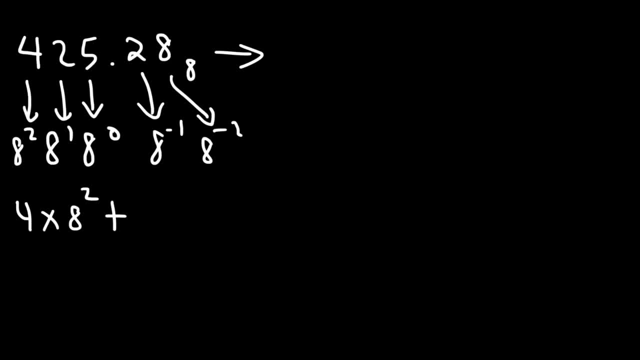 So we're going to have 4.. So we have 4 times 8 squared, plus 2 times 8 to the first power, plus 5 times 8 to the 0 power, plus 2 times 8 to the minus 1, and then plus 8 times 8 to the minus 2.. 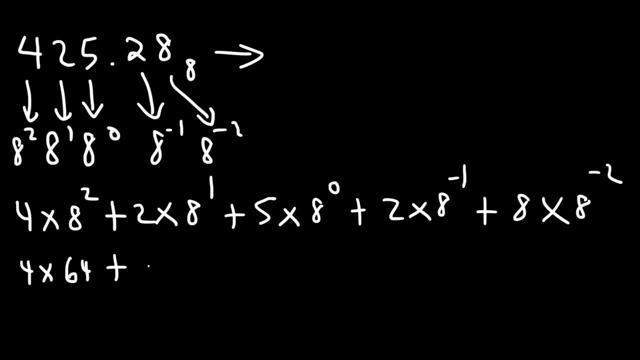 Now we know that 8 squared is 64, and 2 times 8 is 16, and 8 to the 0 is 1,, 5 times 1 is 5.. Now what about 2 times 8 to the minus 1?? 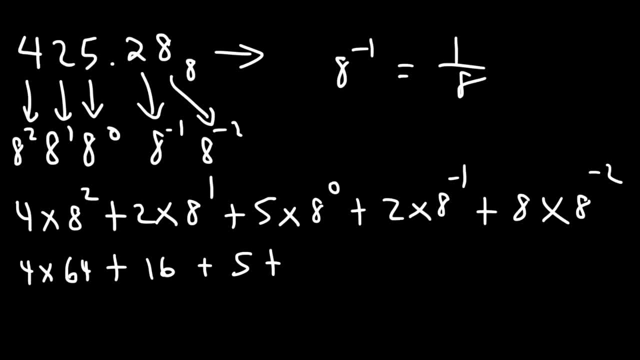 8 to the negative 1 is 16.. That's the same as 1 over 8.. And so, therefore, this expression becomes 2 times 1 over 8, or we could say it's basically 2 divided by 8.. 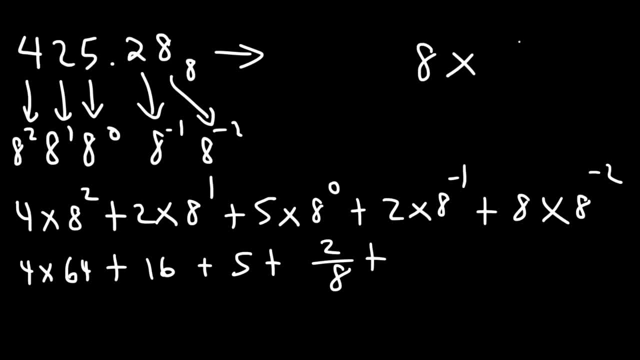 Now for this expression. 8 to the negative. 2 is 1 over 8 squared, And so what we have is 8 divided by 8 squared, which I'll write that here. So 4 times 64, that's 256.. 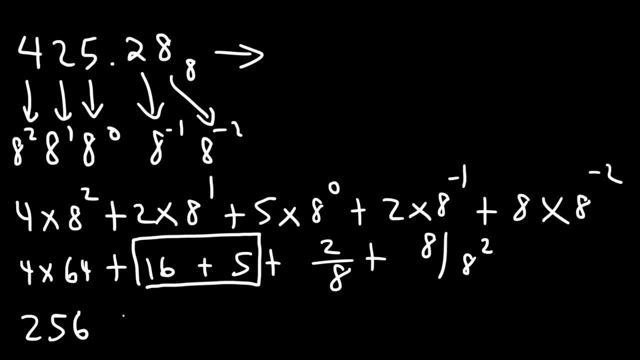 Now we can add 16 plus 5, that's going to be 21.. And then 2 over 8, or 2 divided by 8, that's 0.25.. And then 8 divided by 8 squared, or 8 divided by 64, that's 0.125.